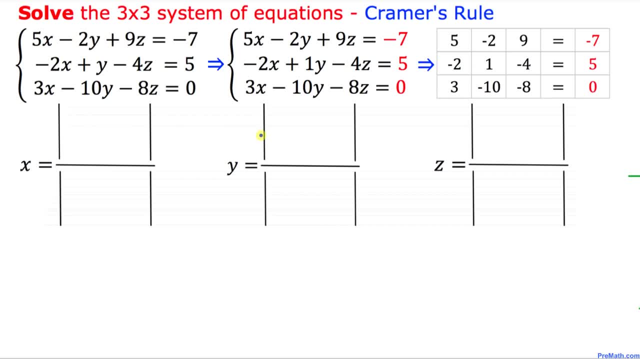 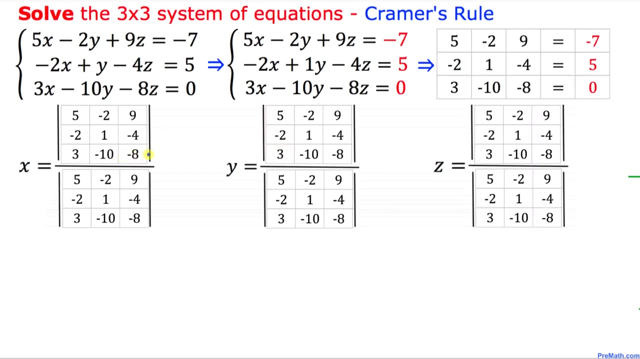 in the next step, we have to start filling out these determinants, these boxes, and let's look at these numbers in this table, on the left hand side of this equation. these numbers are going to go in all of these boxes, all of these determinants, and here, as you can see, we have nicely filled out all these boxes with these numbers. here is 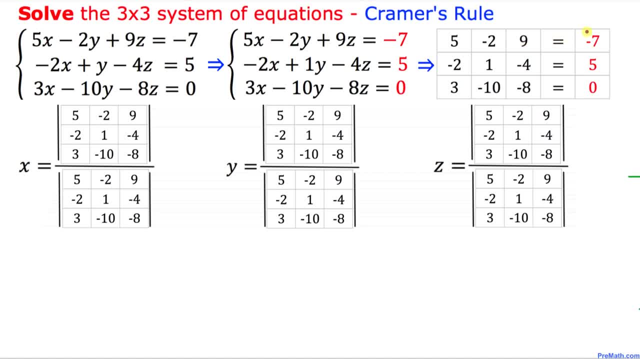 our next step. let's focus on our these right hand side column, these negative 7, 5, 0, these. this column for x is going to go all the way on the left hand side, very first column, as we go along. for y, it's going to shift to the second column right up here and for z is going to be in the 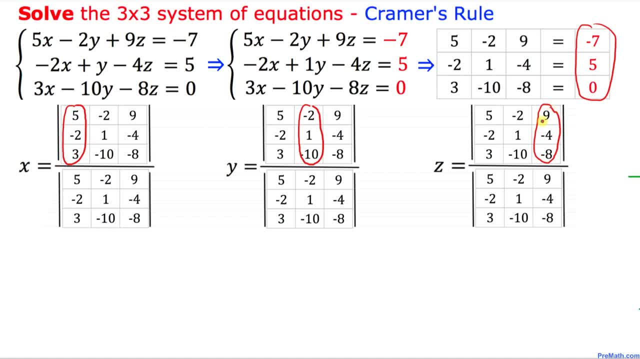 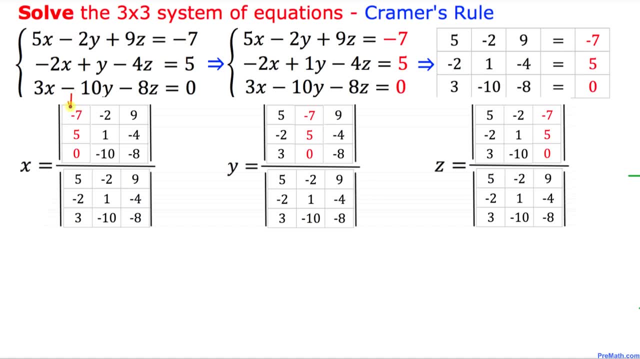 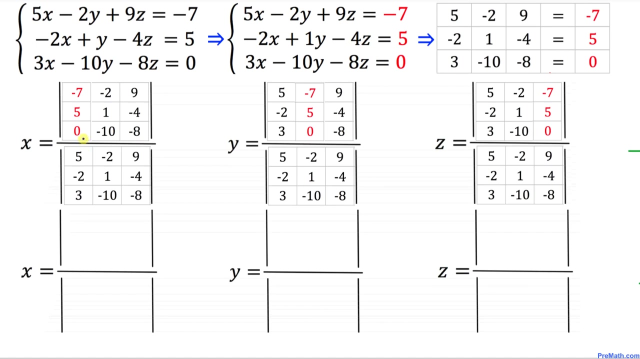 third column for right over here and here are these column for x is the. this red number showed up in the very first column. for y variable it showed up in the second column, on the top. and for z it showed up in the third column. and now let me go ahead and fill out these numbers by: 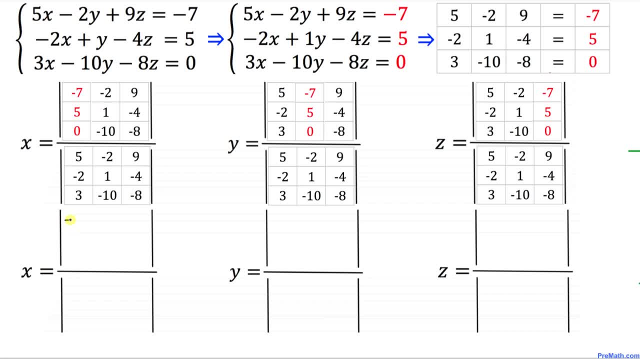 myself. on the top is going to be negative seven, five zero negative two, one negative, ten negative two, one negative ten, nine negative four negative eight. and likewise on the bottom is going to be five negative two nine negative two, one negative four, three negative ten negative eight. and. 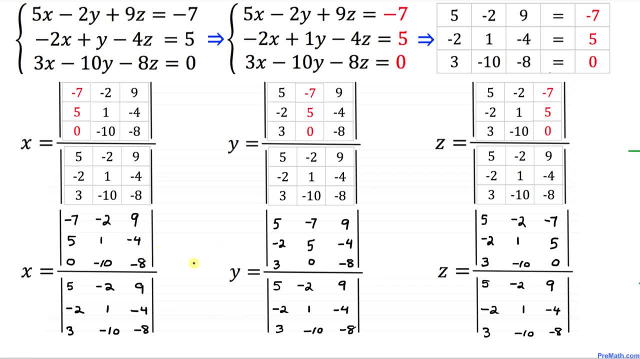 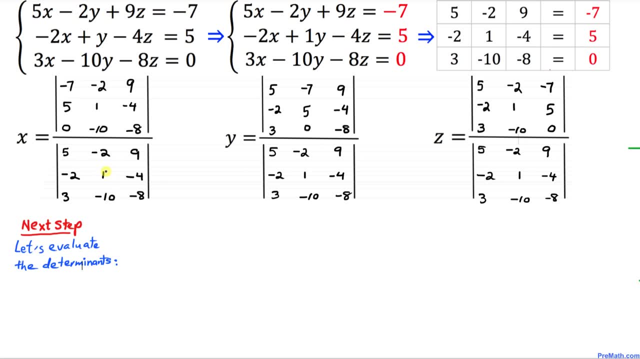 here is our final product after filling out these number. and now, in our next step, we are going to find the value of all these determinants, one at a time. and let's start off finding the value of this determinant for x, at the bottom. and here i have copied down this bottom determinant right up: 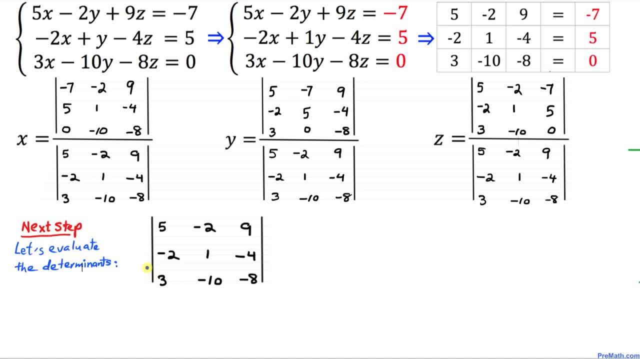 here. let's go ahead and find the value of this determiner. let me show you really easy way to find the value of this determinant. let's draw this horizontal line right above this last row. the very first step is: let's criss-cross, cross-multiply five times. one is five, put a minus sign and negative. 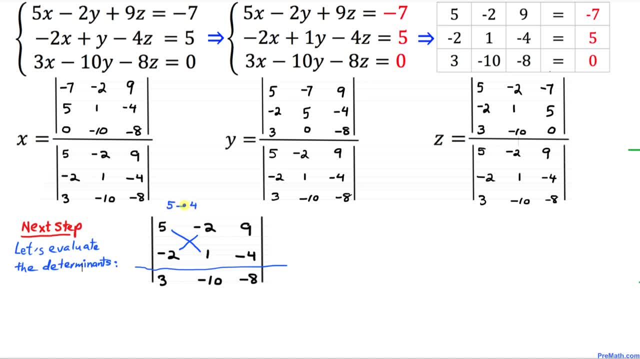 two times negative. two is positive four. always remember you put a minus sign. five minus four is one. this one is going to show up in the right hand side. let's crisscross the next two columns. negative two times negative. four is positive eight. then always put a minus sign and then. 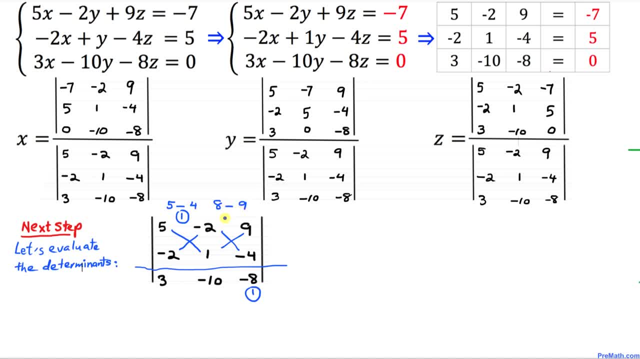 nine times. one is positive. nine eight minus nine is negative one, so negative one is going to go in the opposite direction, as you can see over here. so now the next step is we are going to look at these numbers. 5 negative 2.. let's copy and paste on this side: 5 negative 2, right up here. let's 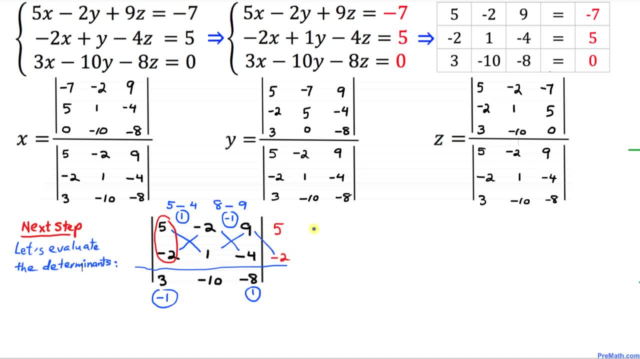 cross. multiply 9 times negative. 2 is negative 18. then put a minus sign 5 times negative. 4 is negative. 20 negative 18 plus 20 is going to be positive 2. this 2 is going to show up in the middle. let's now 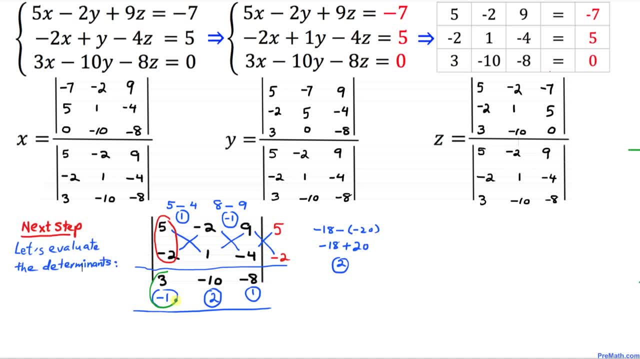 simplify. let's multiply these numbers first and then we are going to add them up. so 3 times negative 1 is negative 3, and then negative 10 times 2 is negative. 20 minus 8 times 1 is negative 8.. If we simplify them, that's going to give us negative 31.. 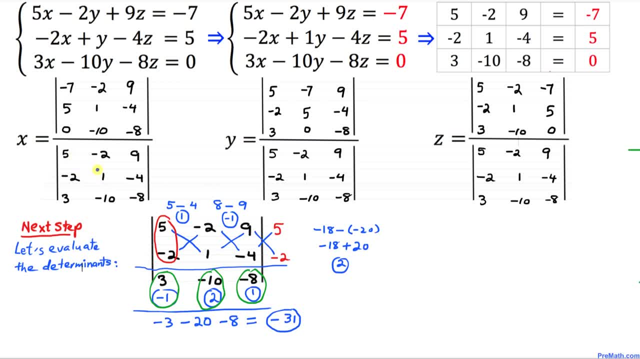 So that means the value of this bottom determinant for x turns out to be negative 31.. And as we can see that all these determinants, these three determinants, are same, so that means they going to have same value- negative 31 for all three of them, negative 31.. And now 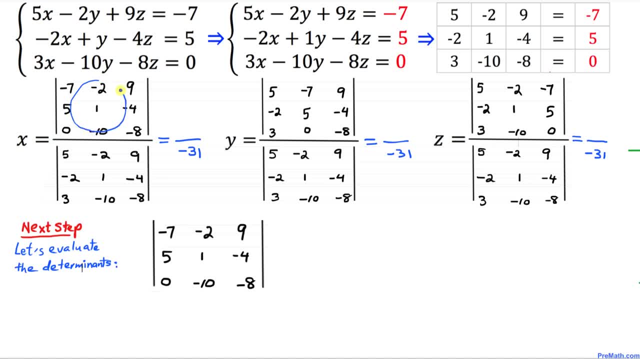 here is the determinant that we going to be finding the value for x on the top is i. here is the determinant that we going to be finding the value for x on the top is i have just copied down. let's go ahead and evaluate this thing once again. we're. 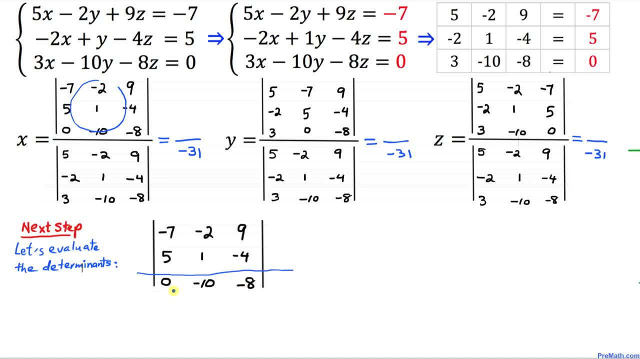 gonna draw the horizontal line above the last row. let's crisscross, let's multiply, cross, multiply. negative 7 times 1 is negative 7. let's put a minus sign and then negative 2 times 5 is negative 10. negative 7 plus 10 is positive 3. this 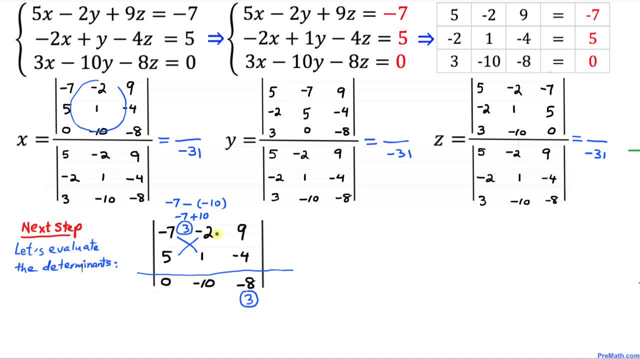 3 is going to show up on this side. let's crisscross the next two columns. so negative 2 times negative 4 is going to be positive. 8 minus 9 times 1 is 9. so that's going to give us negative 1. so negative 1 is going to show up on the 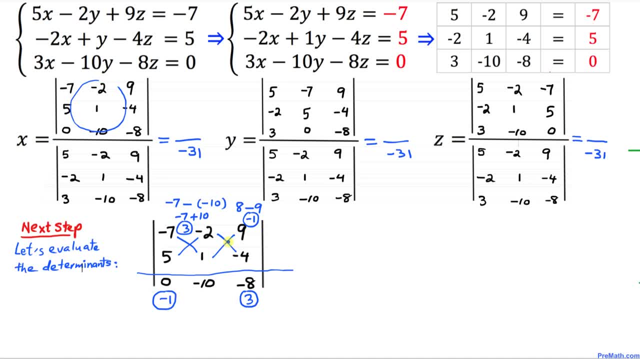 left hand side in the opposite direction. and now let's look at these numbers: negative, 7, 5. I'm going to copy and paste on this side: let's cross: multiply 9 times 5 is 45. then let's put a minus sign: negative, 7 times negative, 4 is 28. that is going to give us simply 17, so 17. 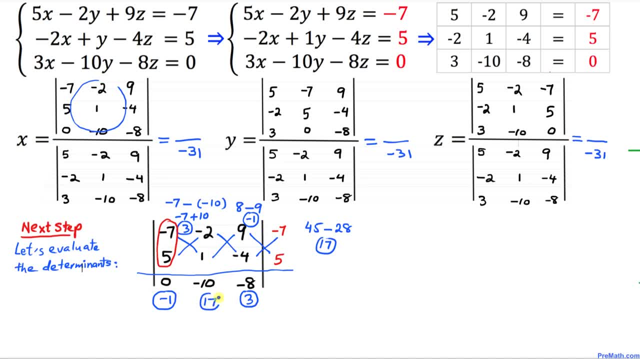 is going to go in the middle. let's go ahead and multiply these numbers faster and then add them up. So if we multiply 0 times negative, 1 is 0 minus 170 and minus 24, and if we simplify that one, that is going to give us negative 194.. So this value is going to show up. 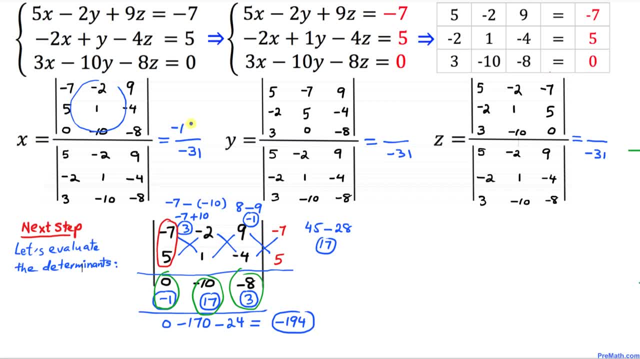 in the top over here: negative 194.. And now we are going to evaluate this determinant on the top, which I have just copied down over here. Let's start evaluating it. Very first thing is we're going to draw this horizontal line right up here. Let's crisscross 5 times 5 is 25.. Put a minus. 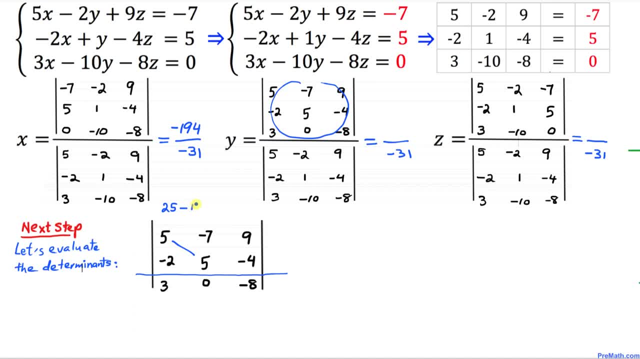 sign. and then negative 7 times negative, 2 is positive 14. So that is going to give us 11.. So this 11 is going to show up in the opposite side right up here. Let's crisscross next two columns: Negative 7 times negative: 4 is positive 28.. Put a. 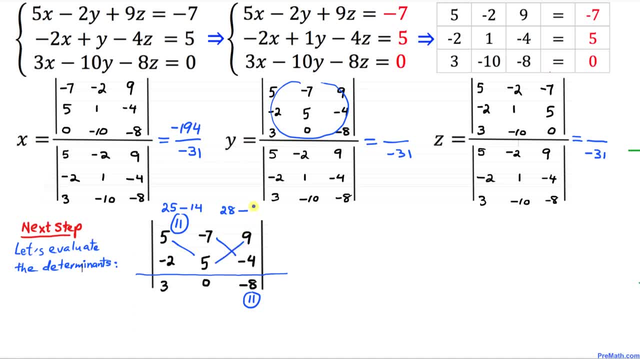 minus sign right before, and this is going to be 9 times 5 is 45 and that is going to give us negative 17.. 17 is going to go in the opposite direction over here on this side. And now, finally, let's look at: 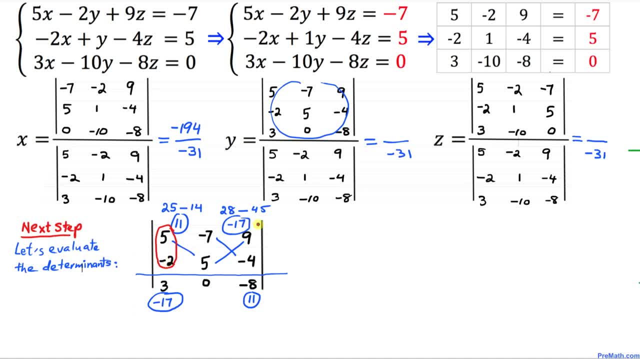 this column: First, column 5: negative 2.. Let's copy and paste on this side and let's cross, crisscross, Cross. multiply 9 times negative 2 is negative 18, and then put a minus sign: 5 times negative: 4 is negative 20.. 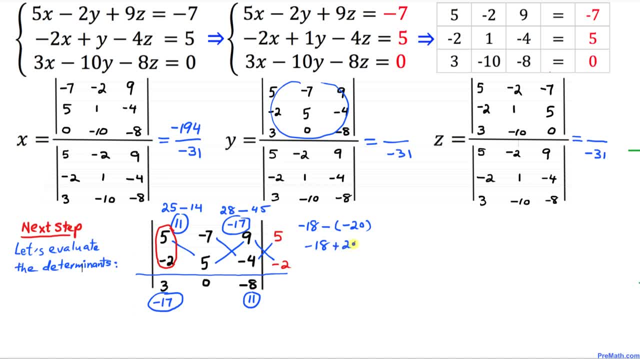 8 negative 18 plus 20 is going to be positive 2 in the middle. right here. Now let's simplify this thing. The very first step is we are going to multiply these numbers first and then we are going to add them up. So 3 times negative 17 is negative 51 and 0 times 2 is plus 0. 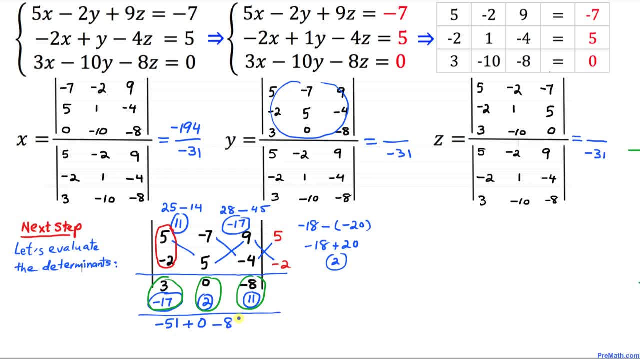 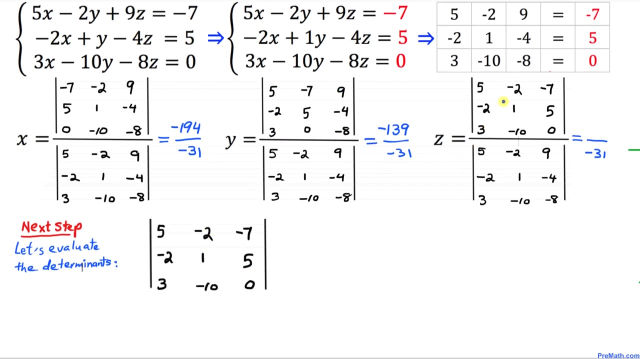 And minus 88. And if you simplify this thing, that is going to give us negative 139.. That means this negative 139 is going to show up right on the top for y variable. And finally, here I have copied down the last determinant, the top part of z, right up here. 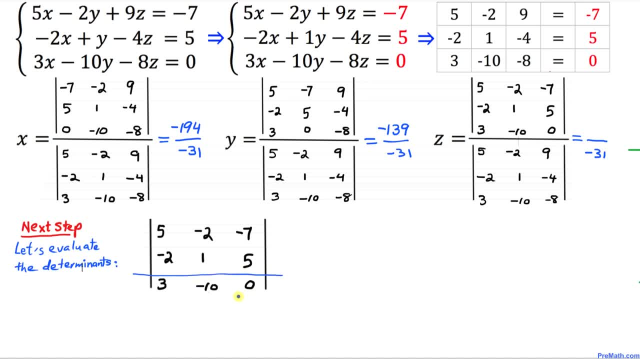 Let's evaluate This determinant once again. we draw the horizontal line first, and then let's crisscross 5 times. 1 is 5.. Put a minus sign. Negative. 2 times negative, 2 is positive 4.. That's going to give us 1.. 1 shows. 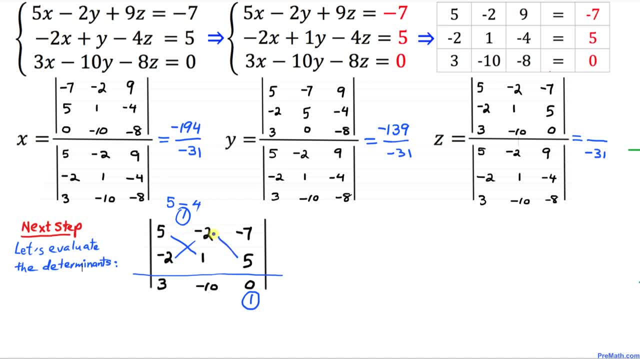 up in the opposite side. Let's crisscross: Negative 2 times 5 is negative 10. Put a minus sign. Negative 7 times 1 is negative 7.. Negative 10 plus 7 is going to be negative 7.. Negative 7 times. 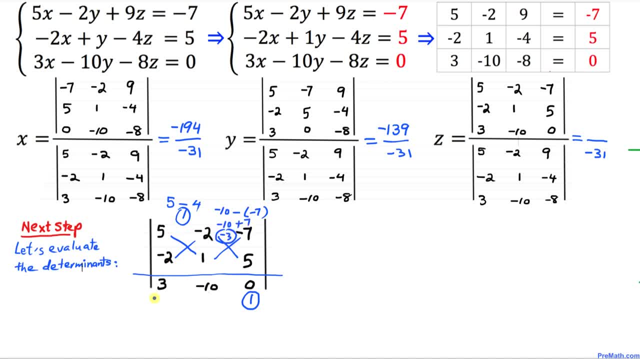 0 is going to be negative 14.. 1 times 1 is negative 1.. Then negative 0 times 3 is positive, 11. It shows up in the opposite side of z, So we have 1 minus negative, 6 plus a negative 5.. 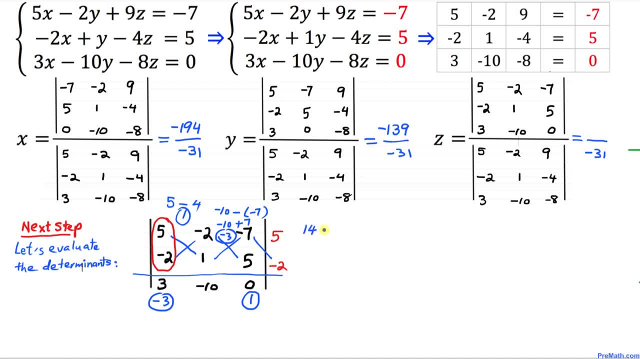 In this situation, each one gives us negative payment. So negative 7 is going to be negative 3 times negative 4.. So this is going to give us negative 7 times negative 2 plus 0. That's going to is going to give us negative 11. that is going to show up in the middle. Let's go ahead and